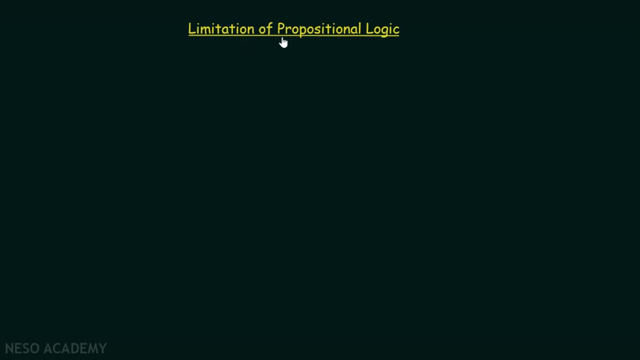 In this presentation, we will deal with one such limitation of propositional logic. So let's get started. The argument which propositional logic can handle is as follows: If it snows today, then we will go skiing. It is snowing today, therefore we will go skiing. 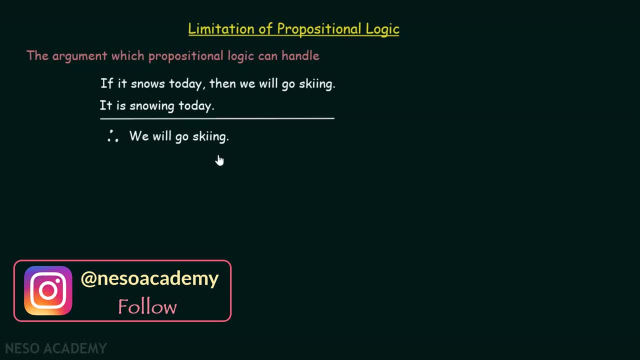 This is an argument which propositional logic could handle easily. Let P denotes it is snowing today and Q denotes we will go skiing, Then we can represent this sentence or this proposition as P implies Q Right. Similarly, I can represent this sentence or this proposition as P. 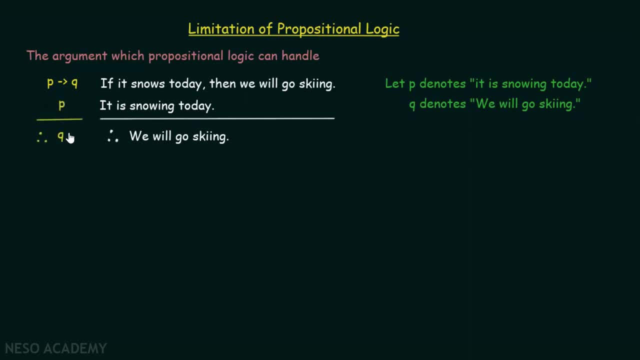 and this can be represented as Q. So I can say the argument will be: P implies Q, P therefore Q. These are the set of premises and this is our conclusion. From these set of premises we can conclude Q very easily by the rule of modus ponens, which we have already seen in the previous lectures. 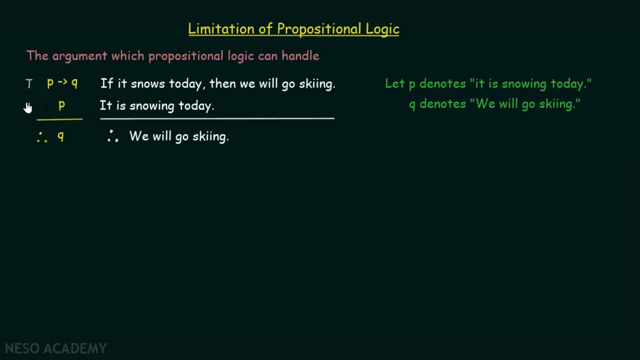 For this we have to let P implies Q is true and P is also true. Therefore, we need to prove that Q is true Here. P is true, therefore Q has to be true. There is no way we can make Q false. 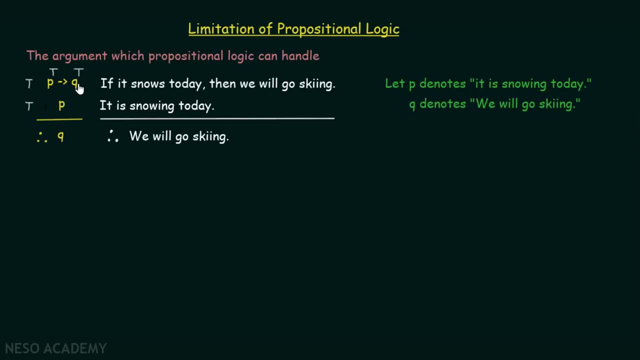 If Q becomes false, then this will be true, implies false. Therefore, P implies Q will become false. That's why it is contradicting itself. Right, We let P implies Q is true, Whenever we are trying to find out the argument is valid or not. 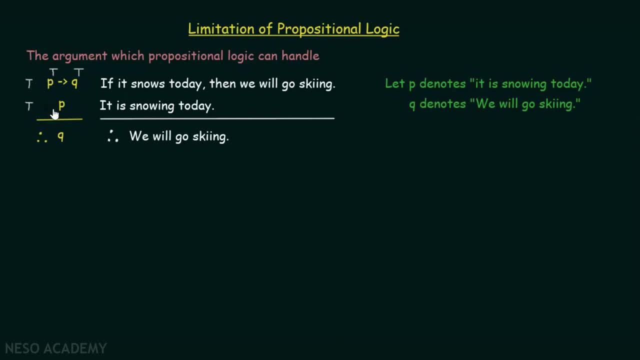 we have to let always that the set of premises are true and therefore our conclusion is also true. We said that P implies Q is true initially and P is also true. If P is true, then Q has to be true. Therefore the conclusion is also true. 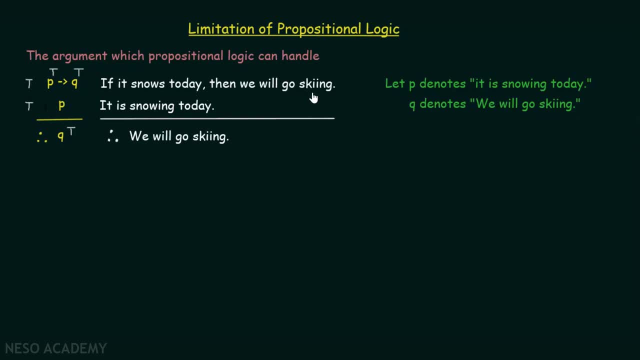 And this is logical as well. If it snows today, then we will go skiing. It is snowing today, then definitely we will go skiing. So this makes sense, right? So this argument is a valid argument. Now, this particular conclusion is true by the rule of modus ponens. 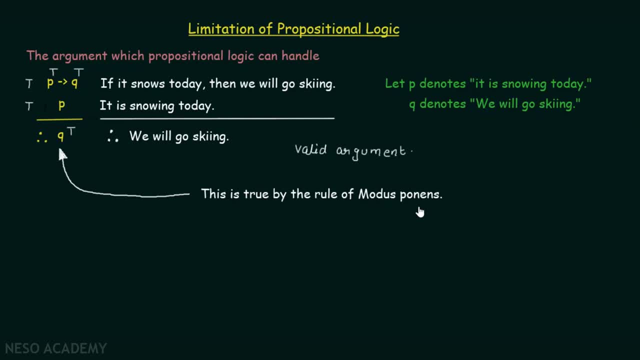 Now let's discuss which type of argument propositional logic could not handle. The argument which propositional logic could not handle is as follows. Here you can clearly see that in this argument I have written: Everyone enrolled in the university has lived in a dormitory. 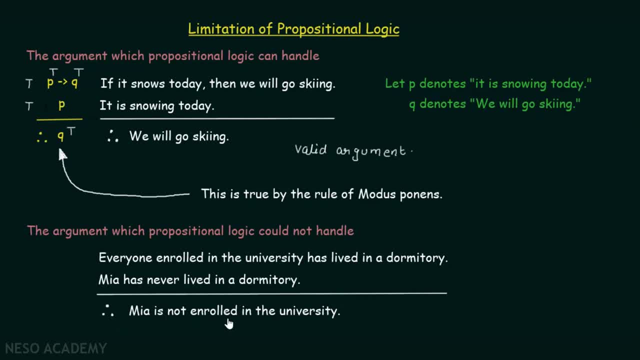 Mia has never lived in a dormitory. Therefore Mia is not enrolled in the university. Now let's see why the propositional logic could not handle such type of arguments. Here you can see that I have written. Everyone enrolled in the university has lived in a dormitory. 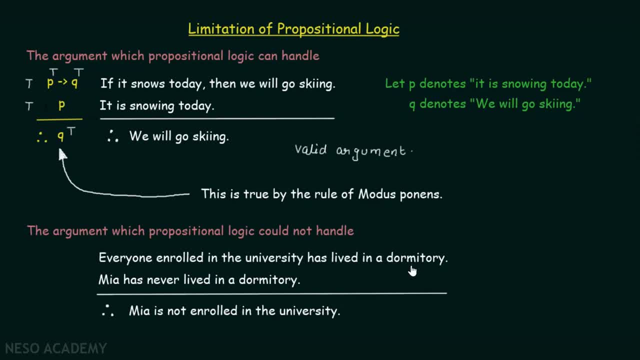 This itself is a proposition. We can't break this down into two propositions right Here. you can see this is: Everyone enrolled in the university has lived in a dormitory. This is a fact. So the person who is enrolled in the university has lived in a dormitory. 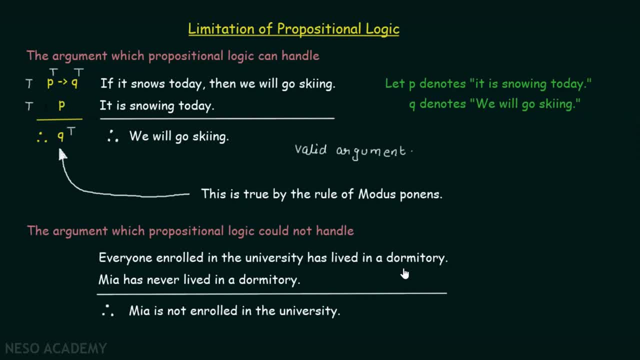 This is a fact. We can't break this down into something like The one part is P, the other part is Q, and make it as P implies Q, right Or P, and Q or P or Q. We can't break this down right. 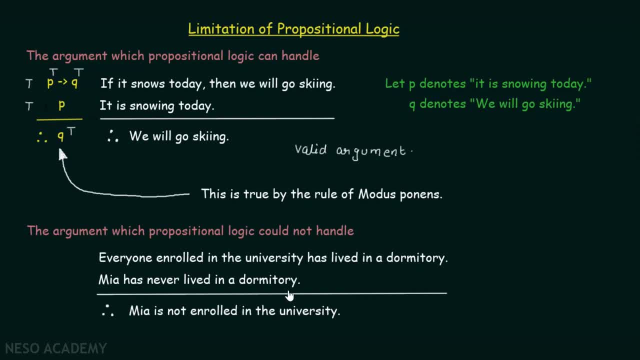 This is itself a proposition. The other sentence is also a proposition, a complete proposition. We can't break this down as well: Mia has never lived in a dormitory. This itself is a proposition, a complete proposition, which is declaring a fact. 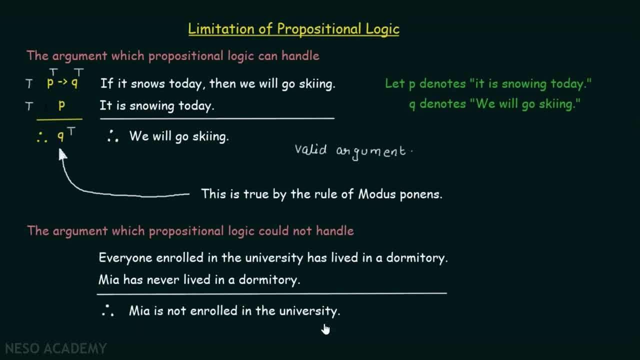 And this conclusion- Mia is not enrolled in the university- is also a proposition, a declarative sentence, a fact, Although if you think logically, then this argument seems correct right Here. everyone enrolled in the university has lived in a dormitory. Mia has never lived in a dormitory. 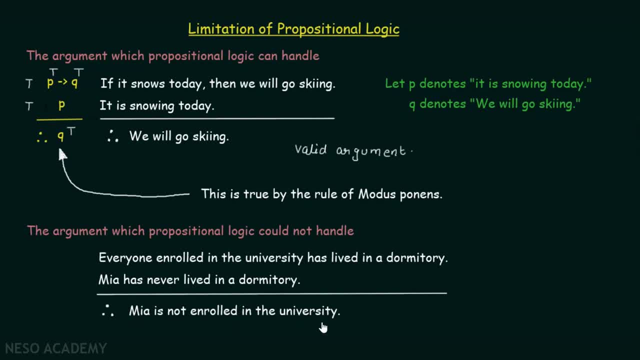 Therefore it makes sense that Mia is not enrolled in the university right. But the validity of the argument needs to be proved with the help of propositional logic, which we can't do here Here, because this itself is a proposition. let's say: this is P. 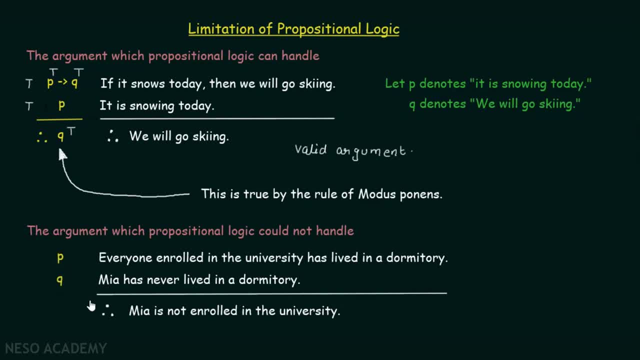 and let's say Mia has never lived in a dormitory? is Q? and let's say Mia is not enrolled in the university? is R- This is the argument so formed. P, Q, therefore R. This doesn't make any sense, right? 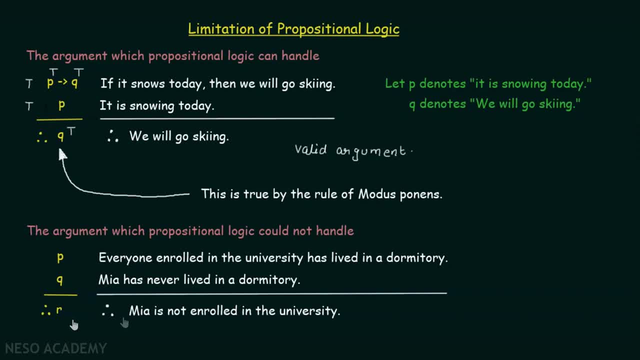 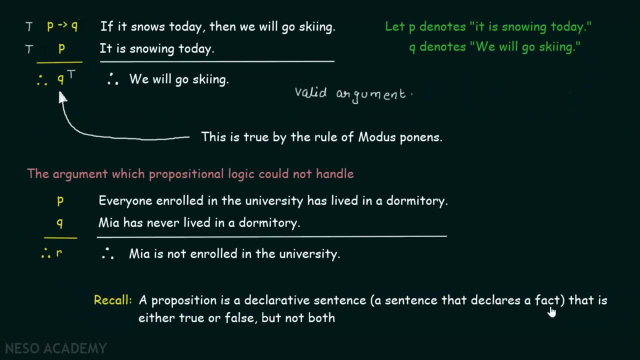 So the propositional logic could not handle such type of arguments. I just want you to recall one thing: A proposition is a declarative sentence, a sentence that declares a fact that is either true or false, but not both. This itself is a proposition.